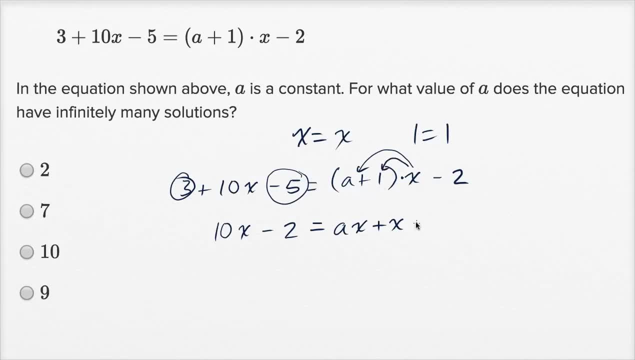 All I did here is I distributed. I distributed the x minus two. Now let's see what happens if let's see I could get rid of both of these negative twos if I add two to both sides. So if I just remember anything, I do to one side. 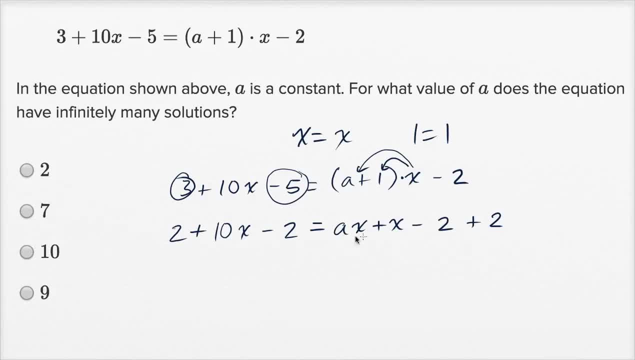 I've got to do to the other one if I want to hold the equality to continue to be true. So I just added two to both sides and I am left with 10x is equal to ax plus x. Let's see, let's subtract x from both sides. 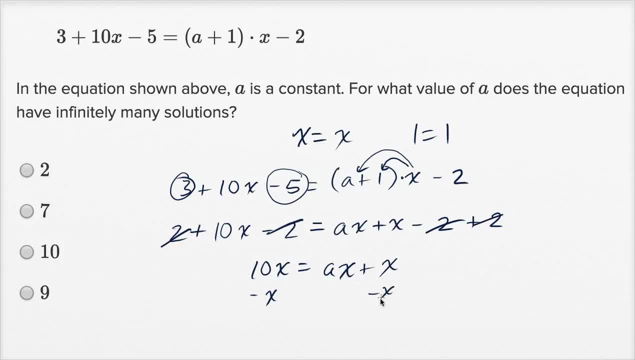 So if I subtract x- actually I could write it like this: I could subtract x from both sides. On the left hand side, I'm going to get nine x. On the right hand side, I'm going to get a, a x. So how could I have an infinite number of solutions? 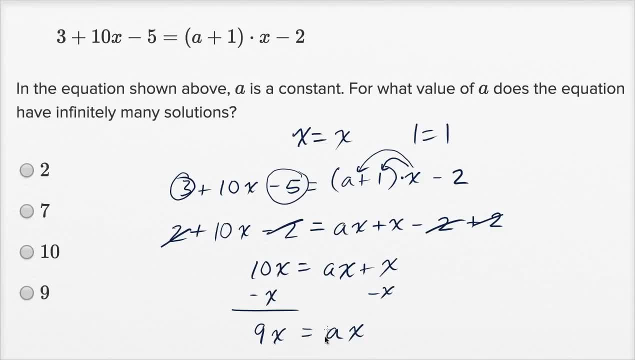 an equation that's going to be true for any x. Well, if a was equal to nine? because if a is equal to nine, I'm going to have a situation. So if a is equal to nine, then you're going to have a situation where nine x. 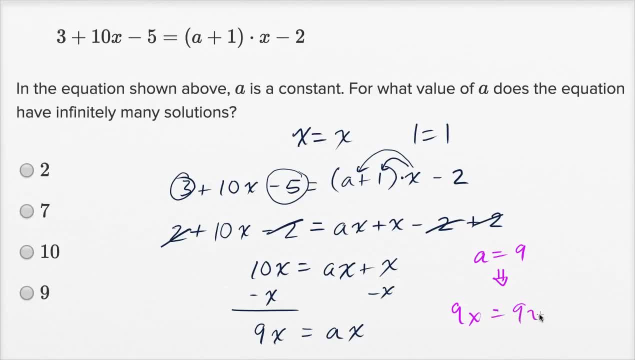 is going to be equal to. instead of a, I'd write: nine is going to be equal to nine x. Well, that's going to be true for any x. Any x times nine is going to be equal to that same x times nine again. 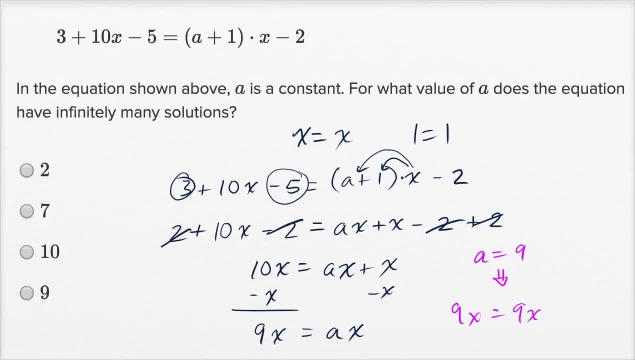 So you're going to have an infinite number of solutions, And so a needs to be equal. a needs to be equal to a is equal to nine. Now, what's really interesting here is think about what would happen if a is any of these. 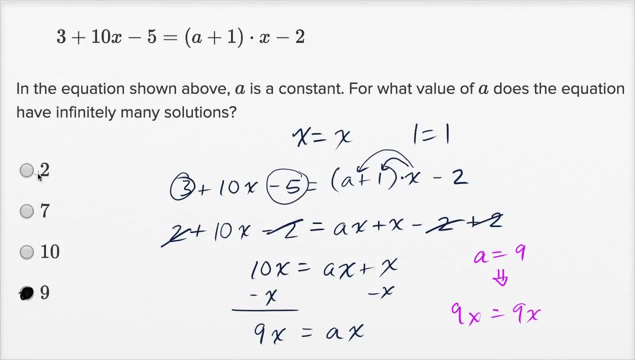 if a is any of these other things right over here, Then you're going to force a different solution. But anyway, we'll leave that for another video. 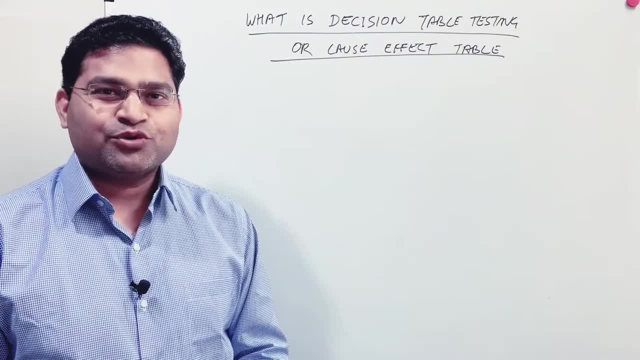 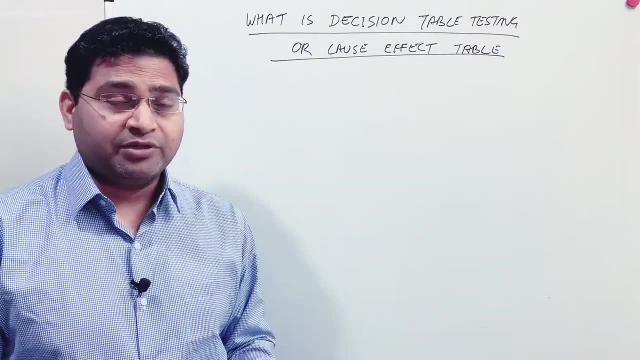 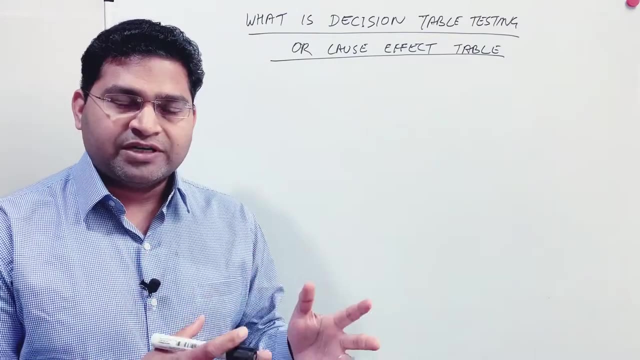 Hello everyone, welcome again. In this software testing tutorial we are going to understand what is decision table testing, or also known as cause effect table. Now, decision table testing or cause effect table, is the software test design technique in black box testing that you utilize. 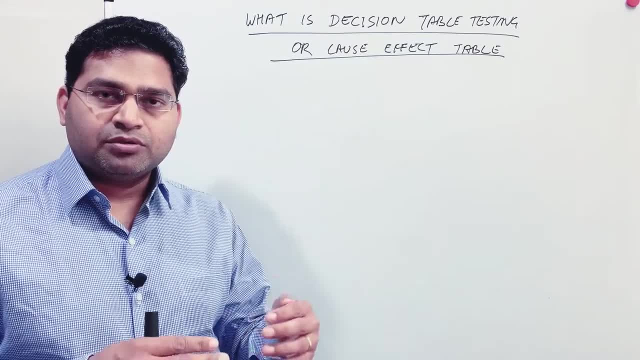 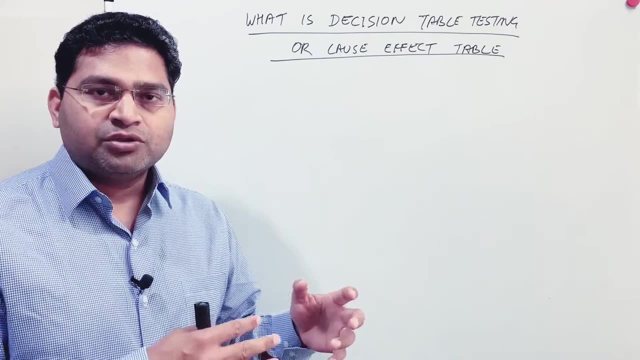 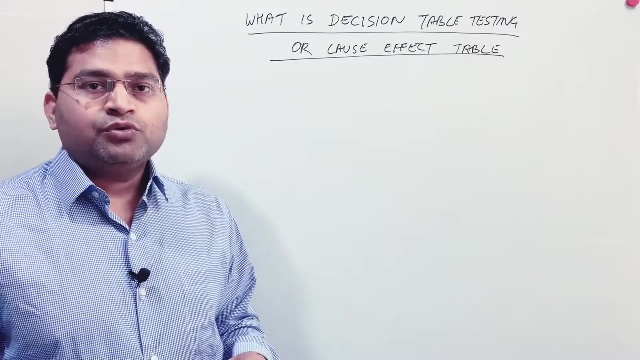 if you have, say, for example, multiple you know outcome or the outcome is based on multiple conditions that are required to test, and this is, you know, very useful in terms of, you know, business rule testing, say, for example. So if you want to test, like in previous examples of